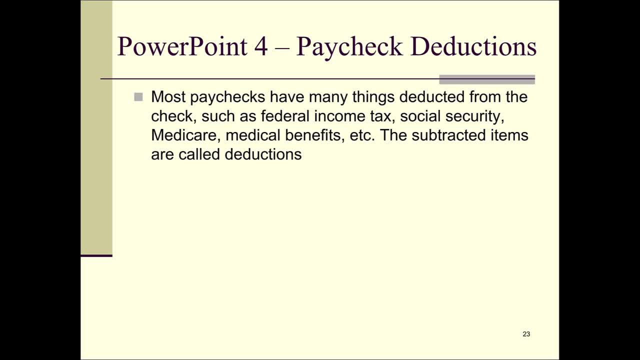 income tax, Social Security, Medicare, potentially medical benefits, etc. The subtracted items are going to be called deductions. So an employee's pay before the deductions is called gross pay or gross earnings. Once you subtract the deductions then you get net pay or take-home pay. It's called take-home. 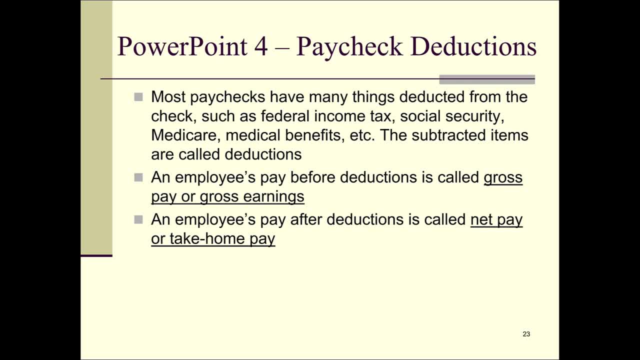 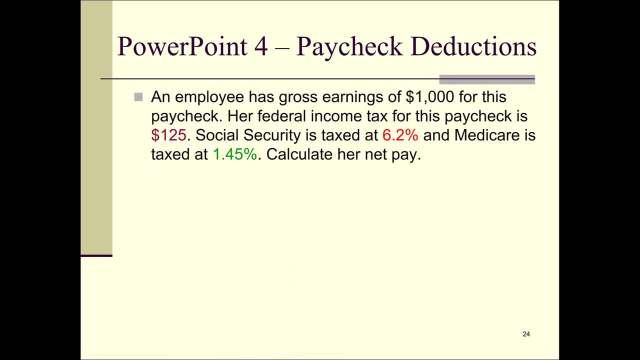 pay, because that's the actual pay that the person gets. Deductions such as Social Security, Medicare, are calculated as a percentage of the gross pay and of course we're going to do a couple of examples. So let's say an employee has gross earnings of $1,000 for this paycheck, Her federal income tax for this. 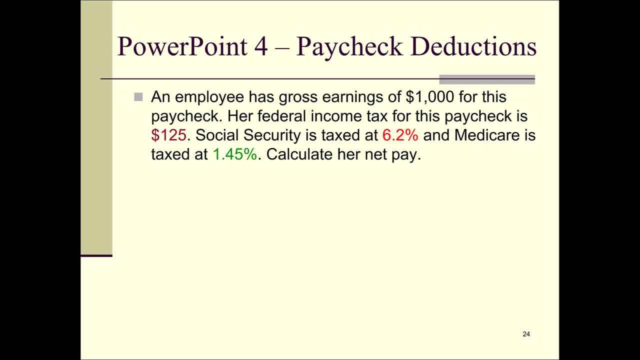 paycheck is $125.. Social Security is taxed at 6.2% of gross and Medicare is taxed at 1.45% of gross. Calculate her net pay. So let's calculate Social Security first. So Social Security is 6.2% of gross pay. So 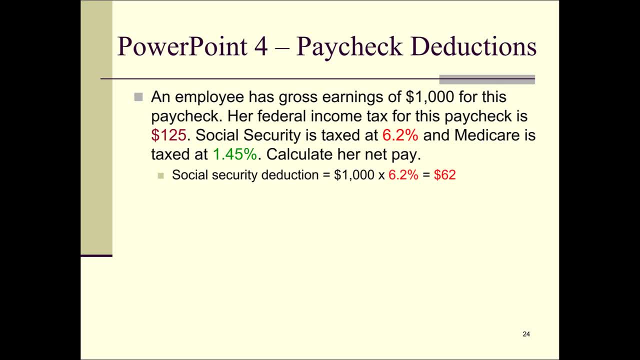 gross pay is $1,000 times 6.2%, so we have a deduction of $62.. Next let's do her Medicare. Medicare is 1.45% of gross, so that turns out to be $14.50.. Next let's do Medicare. Medicare is 1.45% of gross, so that turns out to be $14.50.. 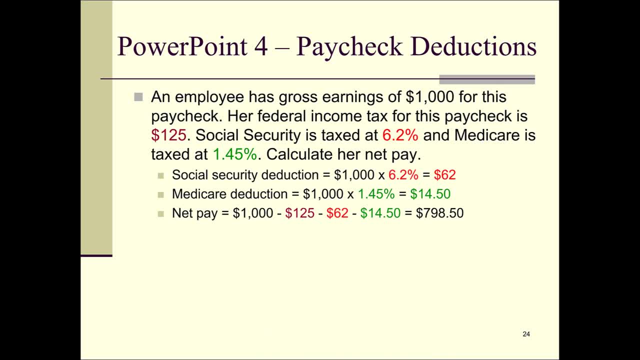 Next let's do Medicare. Medicare is 1.45% of gross, so that turns out to be $14.50.. So her net pay is going to be $1,000 minus the federal income tax of $125, minus the $62 for Social Security, minus. 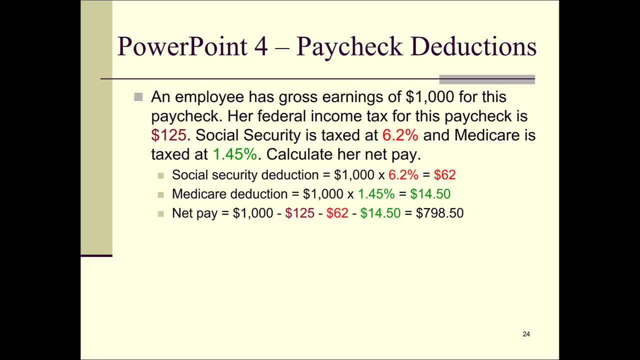 the $14.50 for Medicare gives us take-home pay or net pay of $798.50.. the $14.50 for Medicare gives us take-home pay or net pay of $798.50.. So what's the most efficient way to use our desktop calculator Memory? Obviously, 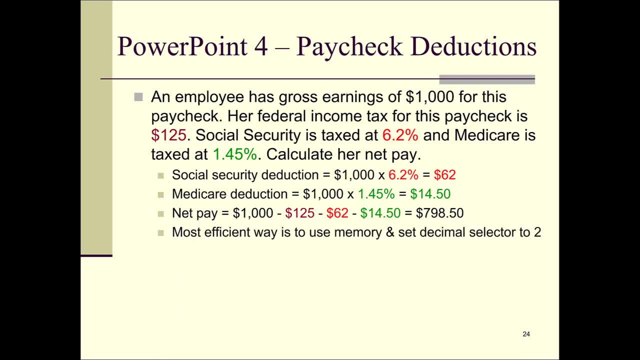 since we're working with currency, you have to set your decimal selector to 2.. So what's the most efficient way to use our desktop calculator Memory? Obviously, since we're working with currency, you have to set your decimal selector to 2.. Because we're going to round to the nearest cent. So the first thing to do, 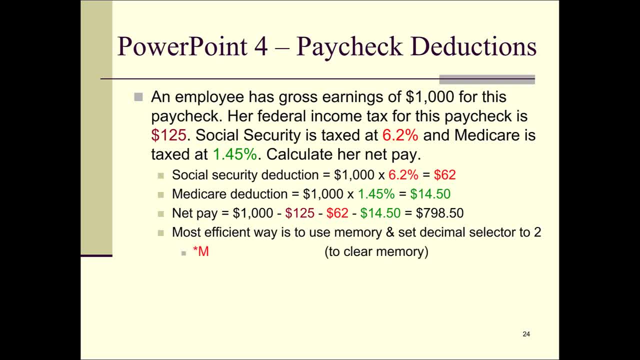 when we're using memory is to clear memory. so asterisk M, and then we're going to add the gross pay, so $1,000 M plus, and then we're going to calculate Social Security and then subtract it. So to do that, enter a thousand times 6.2. 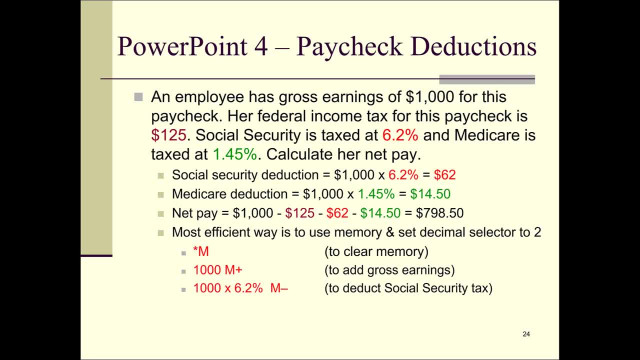 hit the percent sign and then hit M minus, Then we're going to calculate Medicare, So that's a thousand times 1.45 percent M minus. and then we have to subtract the federal income tax, So that's 125 M minus. and then to see what: 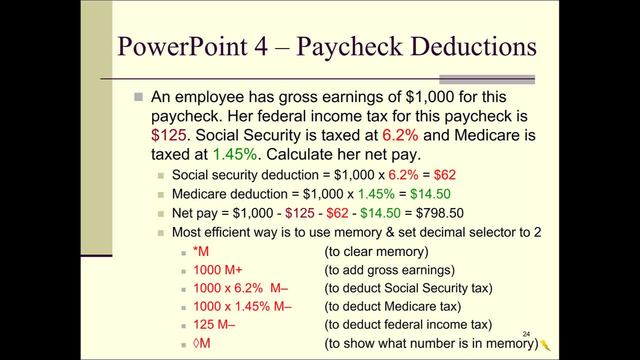 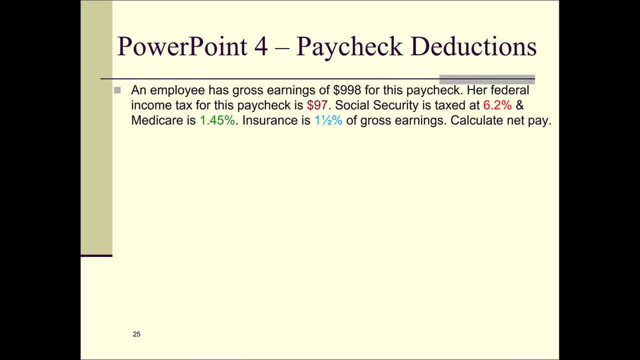 is in memory, hits your diamond M and you should get $798.50.. Let's do another one. An employee has gross or earnings of $998. for this paycheck, Her federal income tax is $97.. Social Security, again, is at 6.2 percent, Medicare 1.45 percent. but they also have 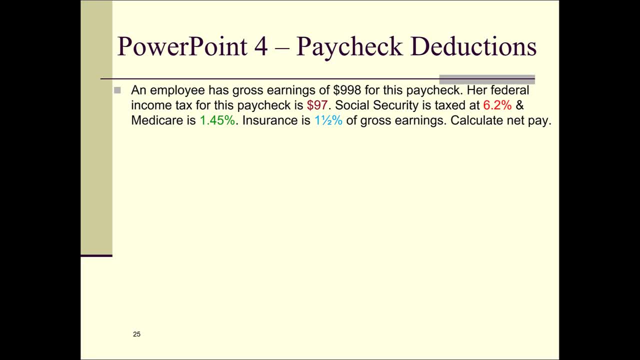 insurance of one and a half percent. So let's calculate her net pay. So let's do Social Security first. Social Security is 6.2 percent, so that's $998 times 6.2 percent gives us a deduction of $61.88.. Medicare is next $998. 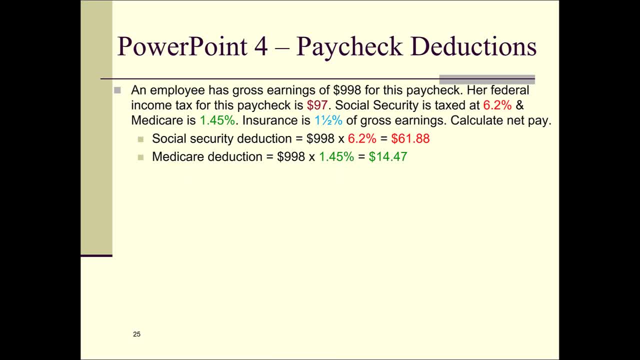 times 1.45 percent gives us a deduction of $14.47.. Insurance is one and a half percent of gross, so that gives us $14.97.. And then to calculate net pay, take gross minus the federal income tax, minus the Social Security, minus the Medicare, minus insurance. gives us a net home. gives us a. 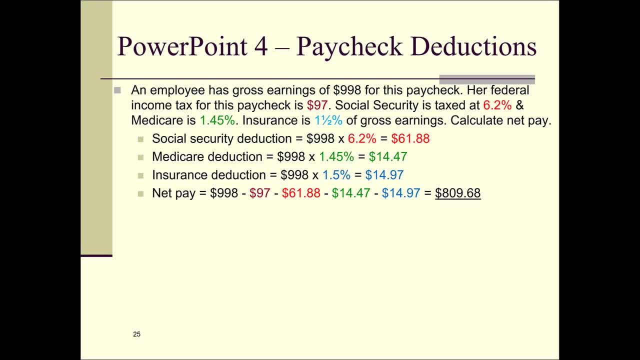 net pay or take-home pay of $809.68.. But let's use our calculator and do this efficiently. Of course, we're still set to two for the decimal selector, so we need a clear memory. asterisk M. Let's add the gross pay to memory: $998 M plus. Let's calculate Social Security: $998 times 6.2.